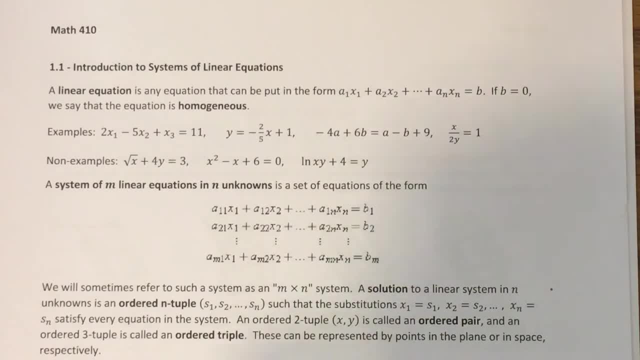 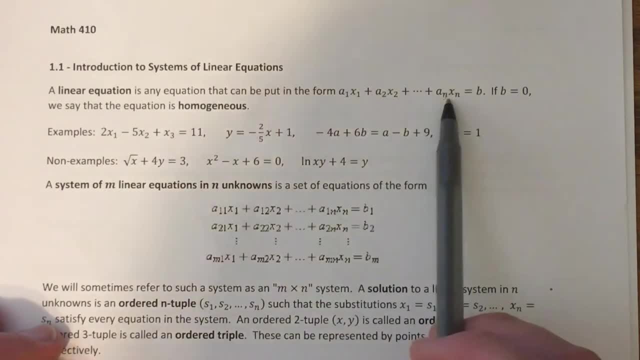 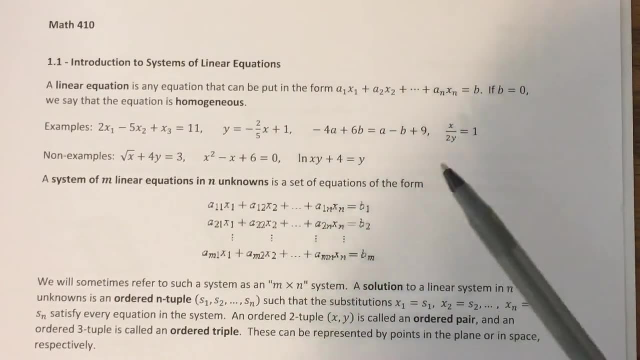 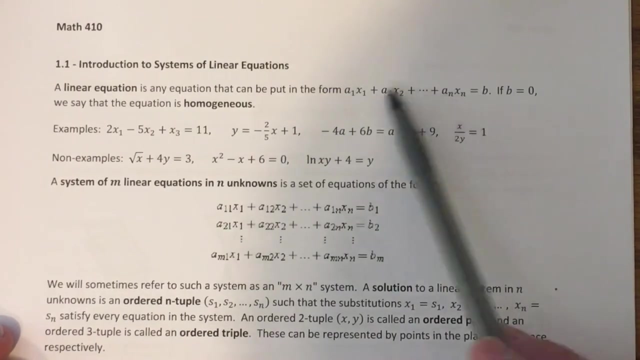 Plus however many terms you know you want until we get to this last one. a and xn equals b. The a's are constants. here the b is also a constant, and the x, the x's are variables. so In the event that b is equal to 0, if this sum of terms here is equal to 0, we say that this: 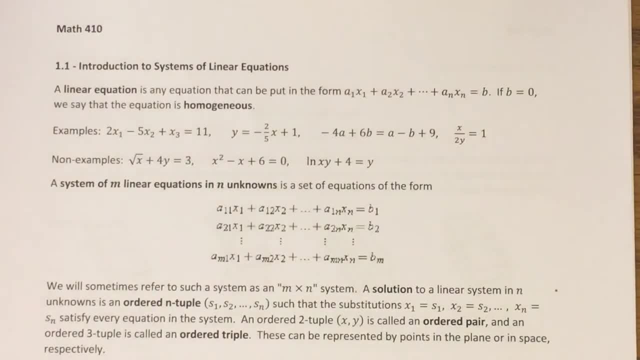 Linear equation is homogeneous. You're gonna see that term a lot in this course. Okay, so here's a few examples- you can look through these- of linear equations. this last one here: You might look at this and think that doesn't look like a linear equation. But try multiplying both sides by 2y and then subtracting the 2y from both sides. you end up with x minus 2y equals 0. 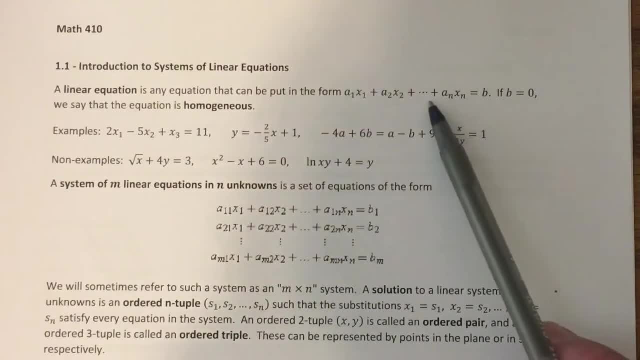 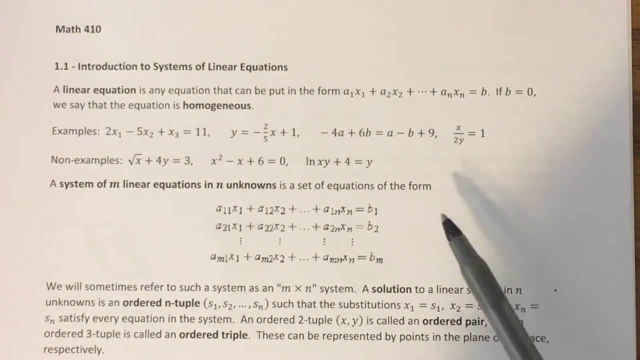 Which is a linear equation because it's, it's the. it can be put into this form and that's the key thing. It doesn't have to start out looking like it's in this form. It just needs to be able to be put into this form to be a linear equation. 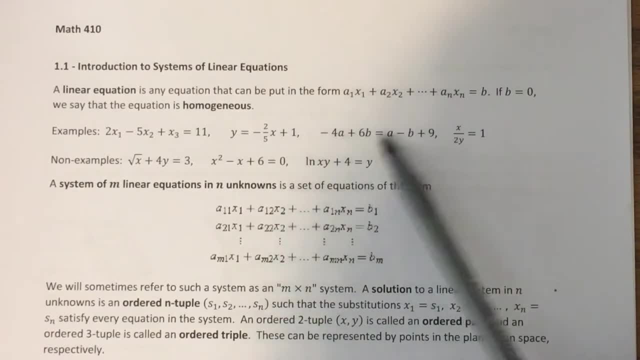 This here is also a linear equation, because If you subtract everything over, or if you subtract the a and add the B over- Let me say it that way- you can combine like terms and you get something that looks like a linear equation. These are non examples of linear equations. 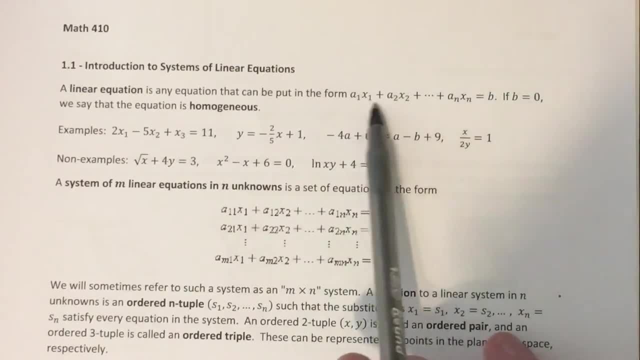 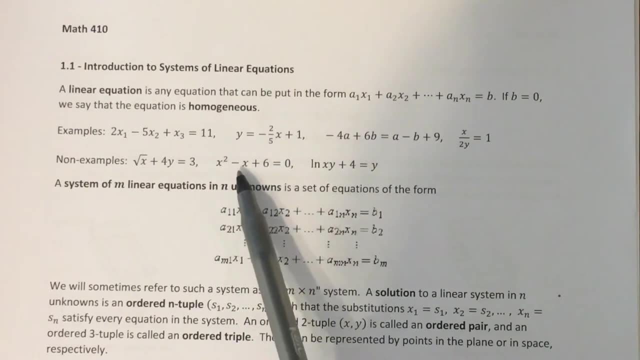 This one has a radical in it, and you'll notice that radicals don't appear in this definition for a linear equation. This one's a polynomial, So the variables in a linear equation cannot be raised to any power other than 1. Okay, even though there can be multiple variables in a linear equation. 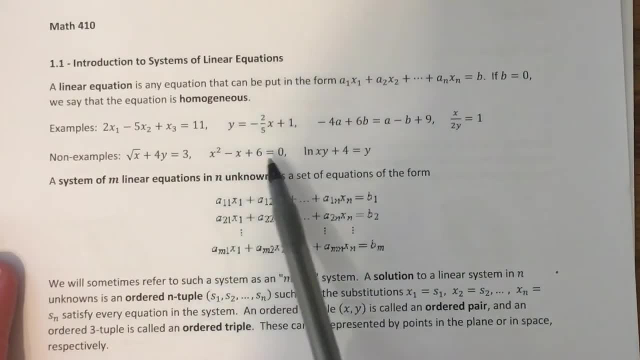 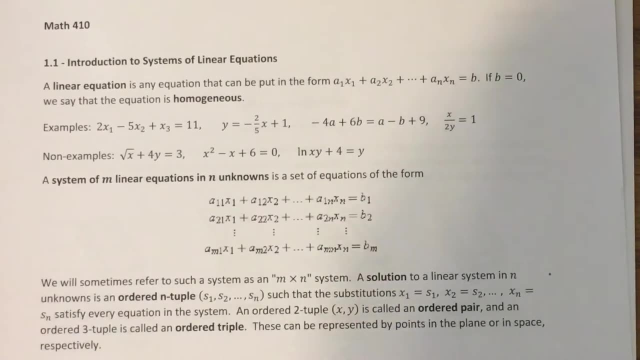 They cannot be raised to any power greater than 1 This one. it has a natural logarithm In it and that's that's not something that can appear in a linear equation. So you know what linear equations are. from algebra that should be. that should feel very familiar. 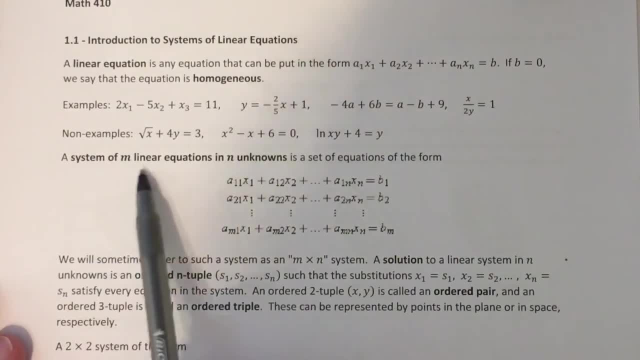 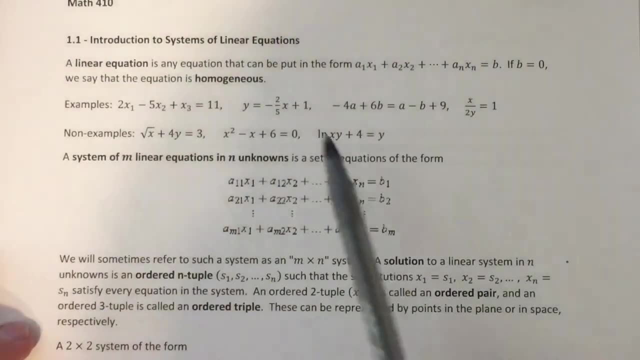 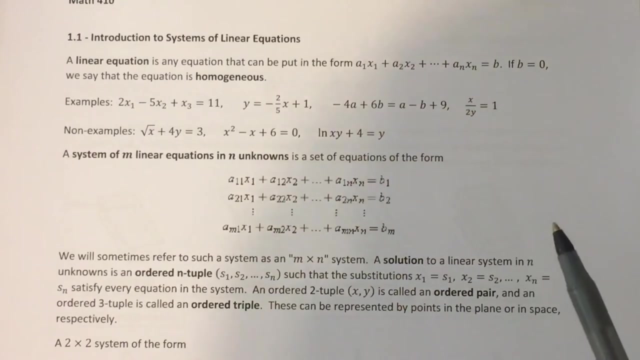 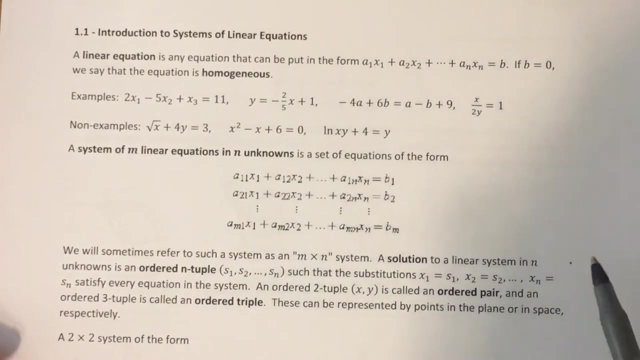 Systems of equations, namely if I say that we have a system of M linear equations in N unknowns, then what we're talking about is M equations of this form in a Simultaneous system. and when I say simultaneous, what I mean by that is A solution to a system has to be a solution that satisfies every equation in that system simultaneously. 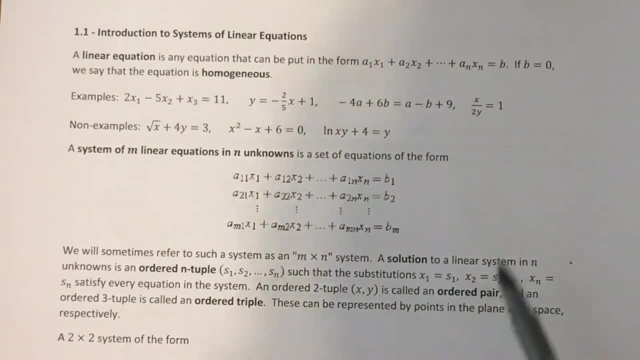 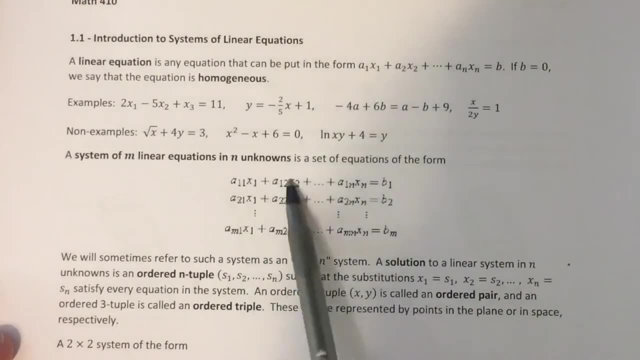 We'll talk about solutions in a moment. So actually we'll talk about solutions right now. this is: this is a general system of equations here And notice the variables I'm referring to as unknowns. I'm usually going to call them unknowns in this class. 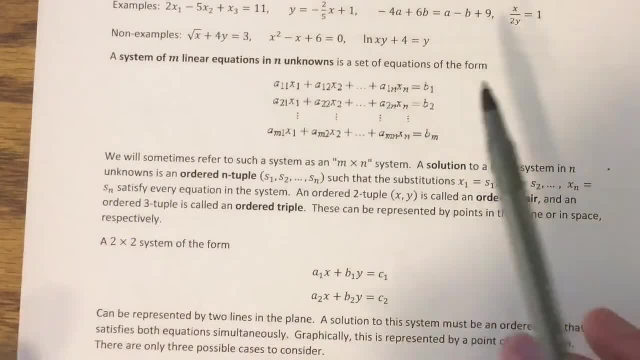 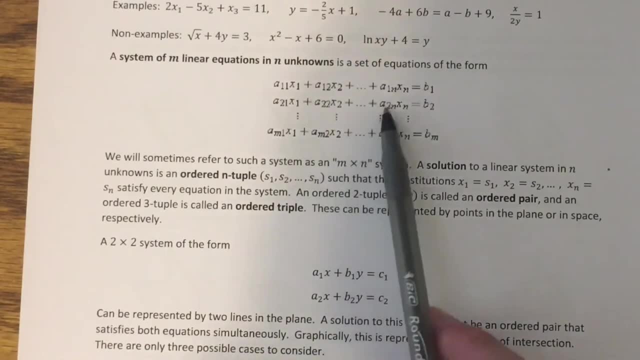 Okay now, oftentimes, because The the topic of systems of equations naturally leads into matrices, We use matrix notation a lot when we talk about systems. in particular, I will sometimes call this system an M by N system, M Meaning the number of equations and meaning the number of unknowns. 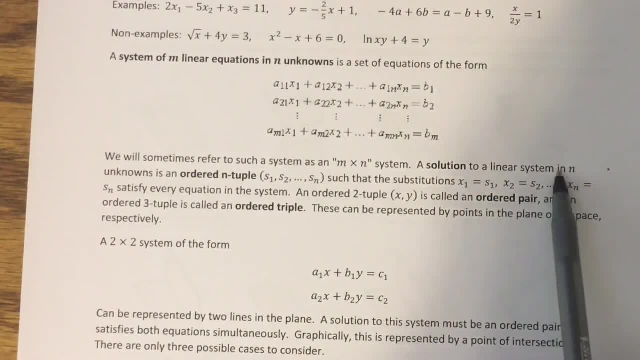 We know from algebra that a solution to a linear system in N unknowns is something that we call an ordered N tuple. So you're familiar with ordered pairs, which I talked about here, ordered triples as well. but because we're being general here, if we have N unknowns in a system of equations a, 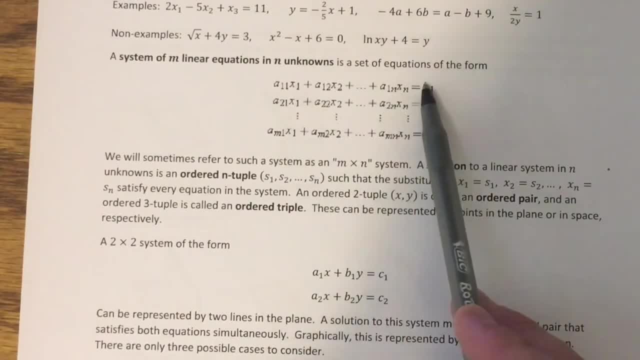 Solution has to provide a value for each of those unknowns that can be plugged into each equation and satisfy that system. So if we put those N solutions into an ordered Sequence like this, we call that an ordered N tuple for whatever N happens to be. Okay. now in the case of ordered pairs or ordered triples, 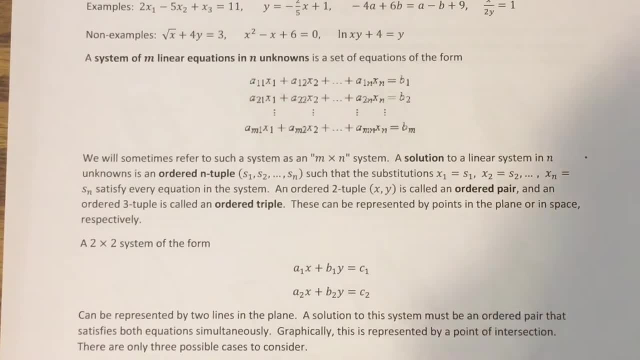 There's some geometry that we can associate with those Ordered pairs. we associate with points in the plane ordered triples. We can associate those with points in space. If you haven't had calculus 3 yet, which you don't need to have had for this class, You may not be as familiar. 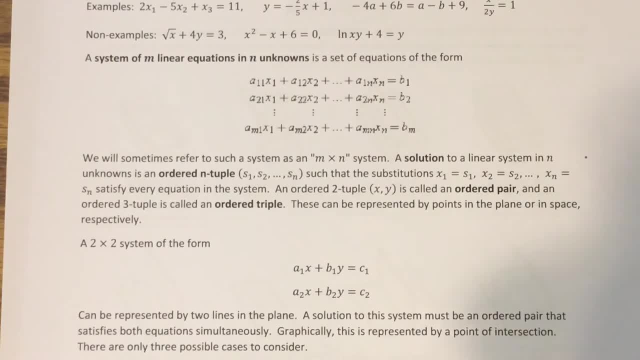 Working in three-dimensional space and you know points and vectors and things like that. We do deal with that in this class And we'll kind of ease into that once we get to that point, But that you can at least imagine an ordered triple as a point in three-dimensional space. 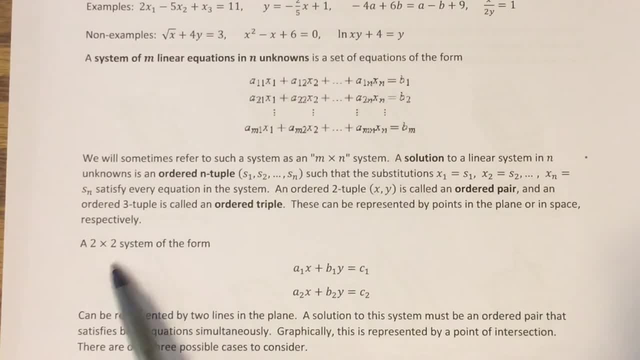 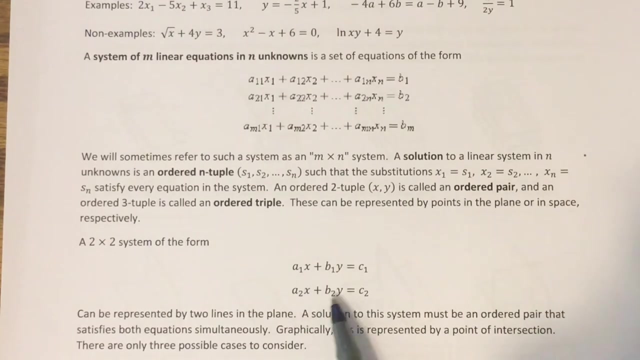 now Let's focus for a moment on just two by two systems, So systems of equations where you have two unknowns and two two equations. here's a general two by two system: a 1x plus B 1y equals C 1. a 2x plus B: 2y equals C 2. 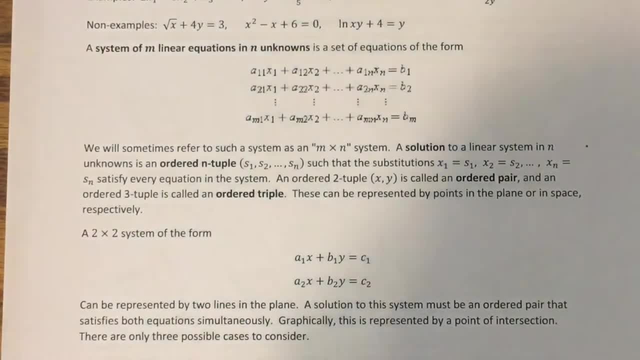 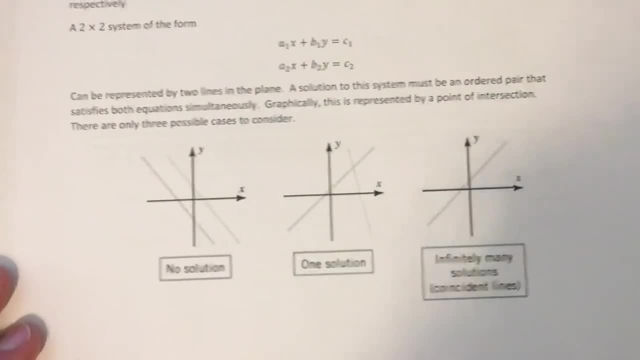 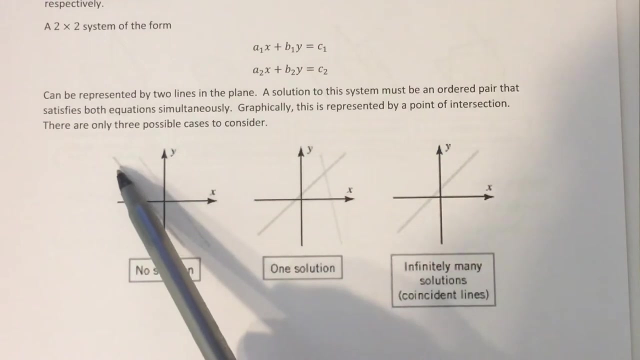 You know again from algebra that linear equations are called linear equations because we can graph them and their graphs look like lines, Which we have some graphs down here, Because systems of two equations in two unknowns are going to be represented by a pair of lines. They're linear equations, So a pair of lines in the plane. We have a few different cases We can look at in fact. 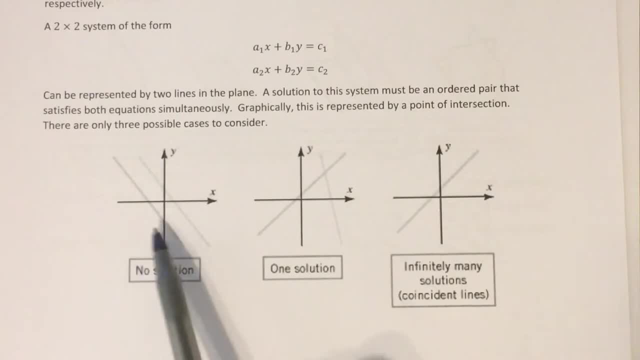 There's three specific cases That we're gonna break this down into. so, first of all, Remember, a solution to a system of linear equations has to be, in this case, an ordered pair, because we have two unknowns, and it has to satisfy both equations Simultaneously. but what is the graph of an equation? Well, the graph of an equation is just the set of all. 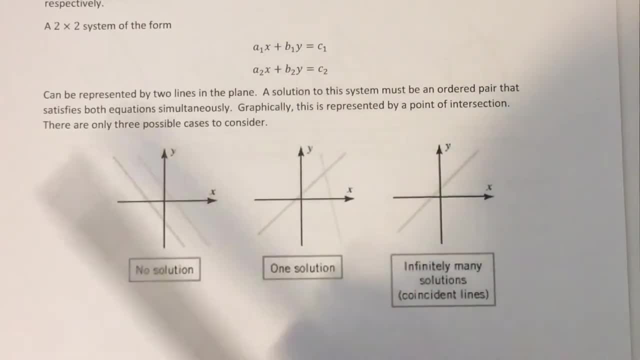 points, in this case ordered pairs that satisfy that equation. so graphs, in this case of lines, are visual depictions of solution sets for an equation. Now, if we're looking for a solution to a system, we're looking for a simultaneous solution, which means we need to find a point. 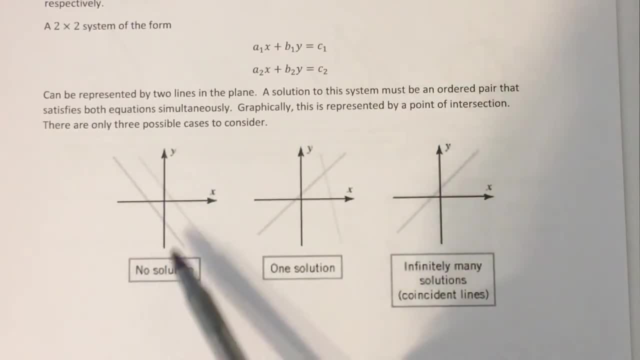 That's on both lines simultaneously, and Graphically it's easy to see where two two lines would contain The same point. we call that a point of intersection. So here, if the two lines represented by the system of linear equations are parallel, Then the two lines will never intersect and that would mean that they have no solution. There's no point that they have in common. 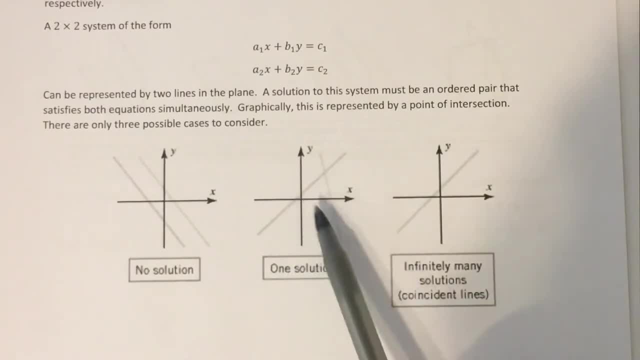 if you have two lines that have different slopes, like this, and they're guaranteed to intersect at exactly one point. so, So in a case like this, we can have one solution to our system of linear equations. The only other possible case for a system of two equations and two unknowns is that the two lines are in fact the same line. 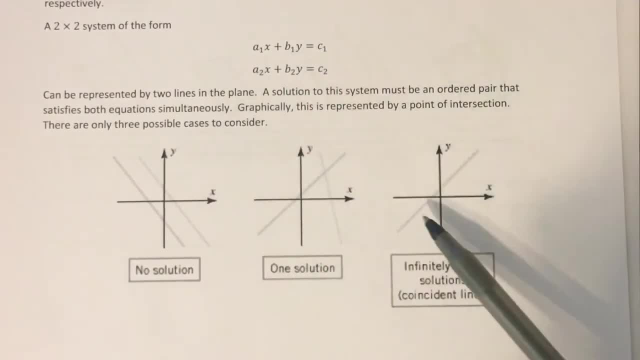 These equations can actually look slightly different from each other, but their graph can still be the same line. In those cases, we say that the two lines coincide, or we call them coincident lines, and every point on either line is a point of intersection. 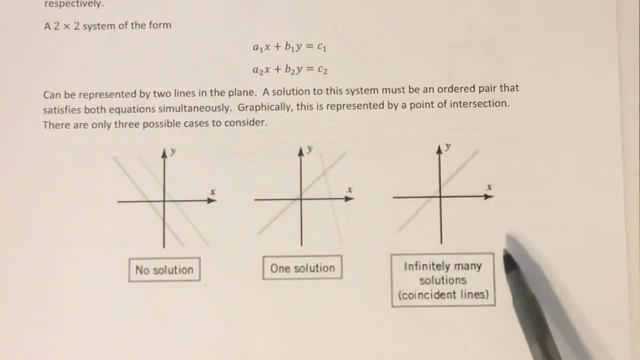 So every point on that line is a solution to that system of linear equations. In those cases we have infinitely many solutions. Be careful with this, because to say that a system has infinitely many solutions does not mean that every ordered pair is a solution, Only the ordered pairs on that line. 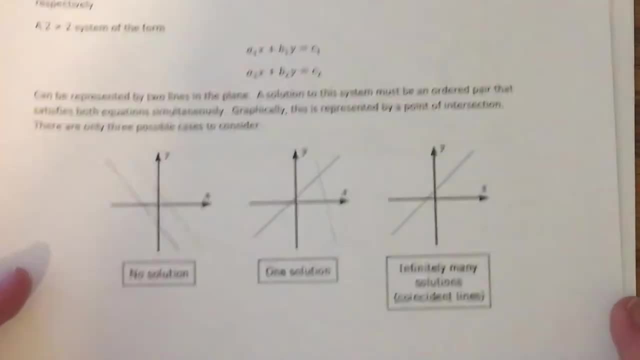 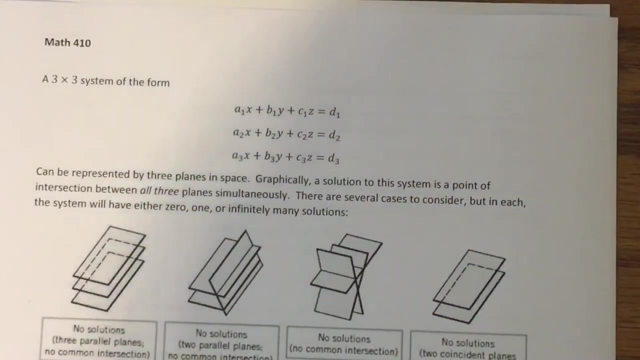 but there are infinitely many of those. Okay, So with that, let's take a look now at three by three systems. And again, if you haven't had Calculus 3, you may not be as familiar working in three-dimensional space. 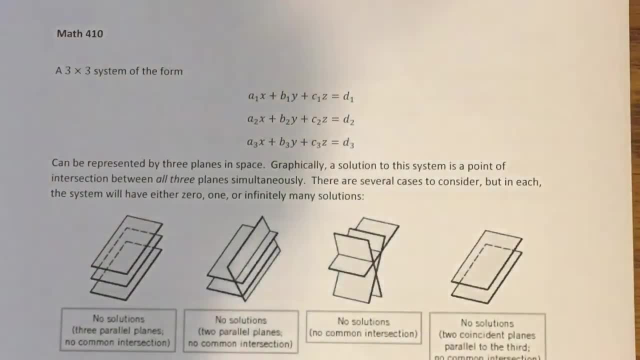 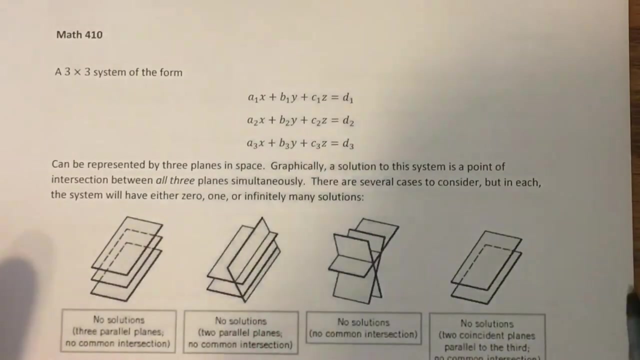 So some of these things you're gonna have to just take my word for it. but whatever the case, this is what a general three by three system would look like. Now, in three-dimensional space, a linear equation actually doesn't look like a line. 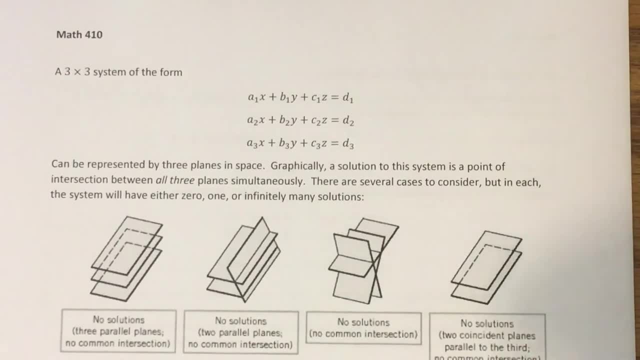 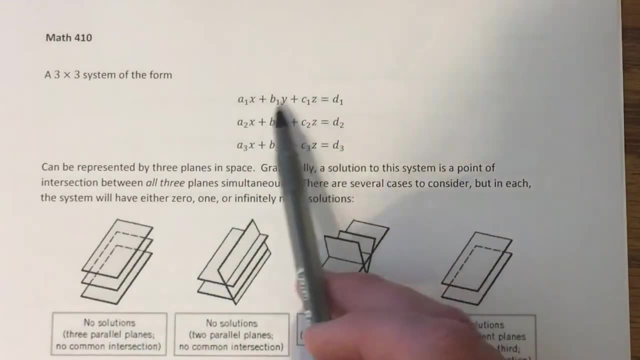 We can graph lines in three-dimensional space and we're going to talk about how to do that in chapter three. But even though it's called a linear equation in three variables like this- x, y and z- the graph of this equation actually looks like a plane, not a line. 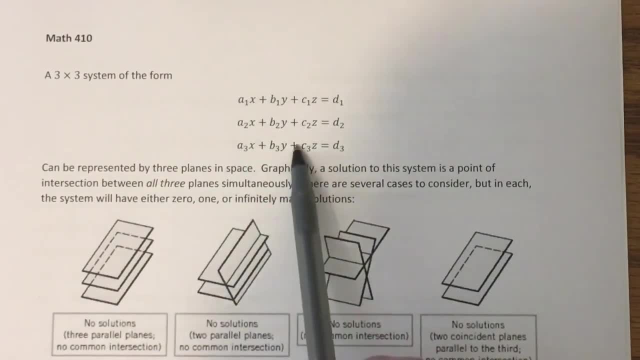 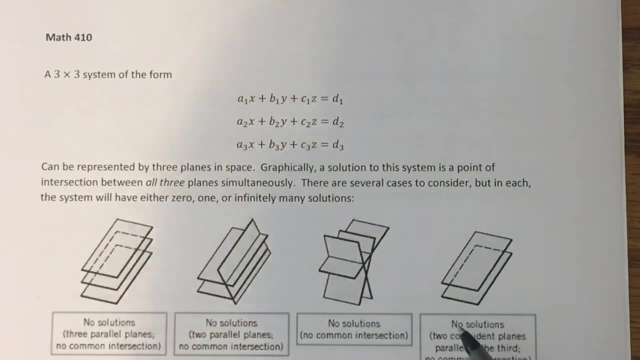 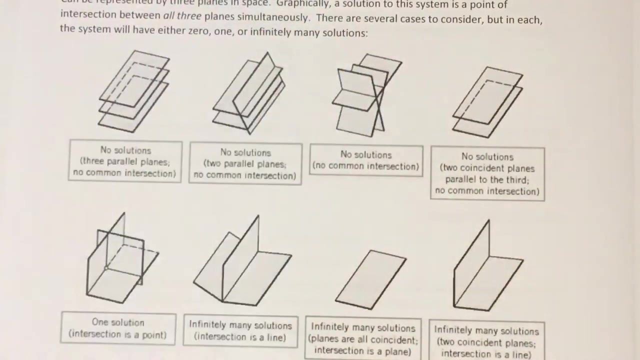 So when we're talking about a system of three equations in three unknowns, then we're talking about three planes, if we want to look at them graphically. So, just like with the case of lines in the plane, if we're looking for solutions to a system like this, then we're looking for. 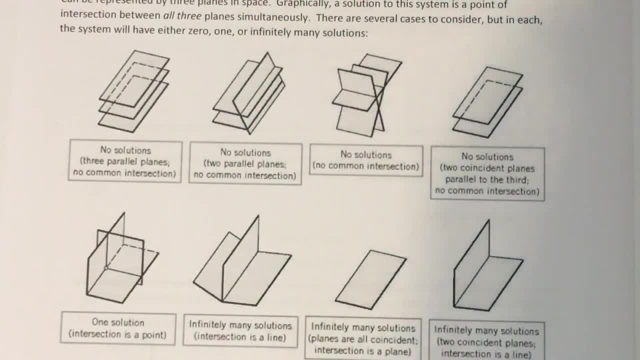 points of intersection between three planes. Now, with planes, there's a lot more different cases to break this down into, but it turns out that, even though you can look at all these different configurations for the three planes, it actually boils down to the same. 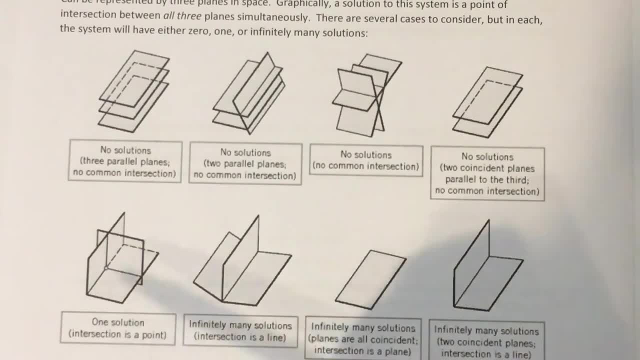 same three categories in the bigger picture. So, for example, in this case here we have three parallel planes. None of the three planes intersect with any of the others. so there's no hope of having a solution to this system because there's no common point. 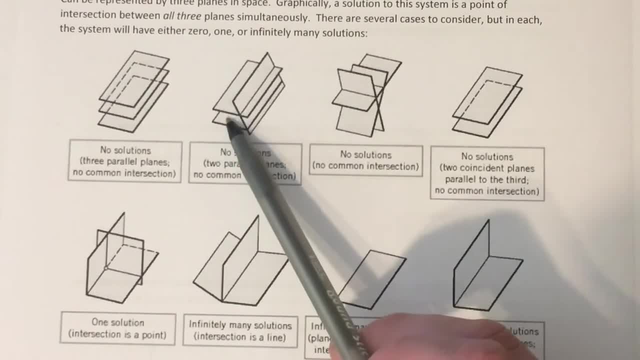 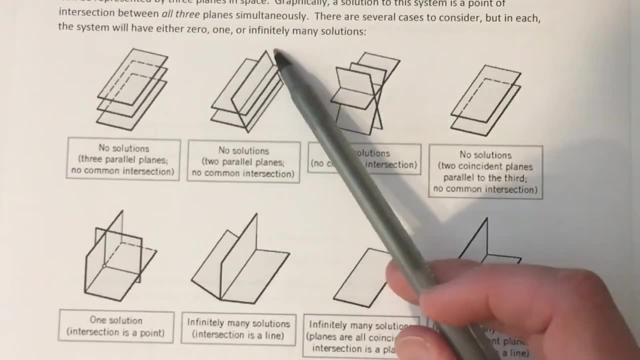 Here we have two parallel planes and another plane, the third plane, that cuts through both of those. This has no solutions either, because even though this plane intersects the other two for a system of three equations and three variables, like what we have up here, 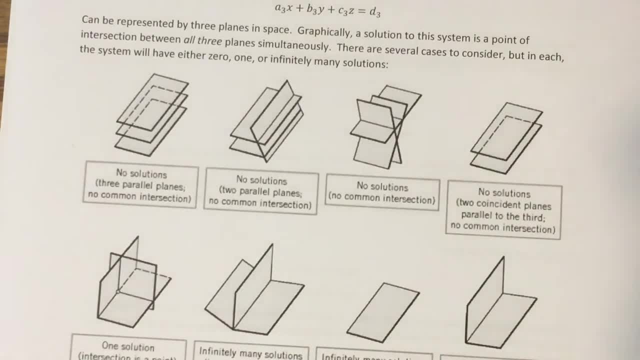 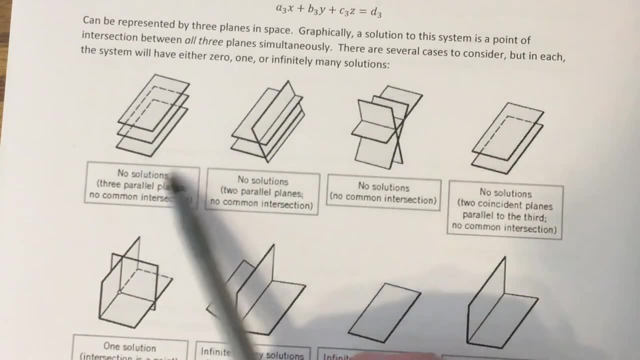 we need a point that's on all three planes at the same time. So an intersection between two of those planes is not enough. it needs to be an intersection between all three. Everything in this top row are examples of where we have two. Everything in this top row are examples of where we have two. 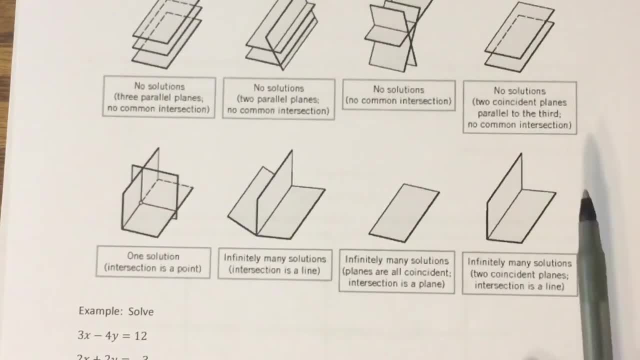 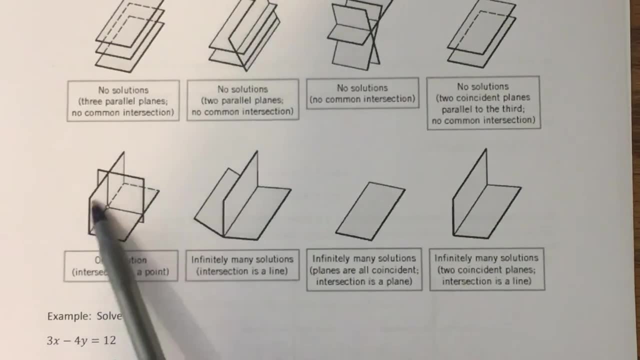 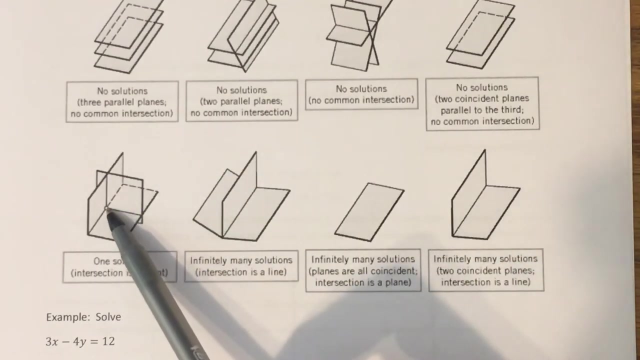 have no solutions at all Down here. we have some cases where we do get some solutions Here. these three planes intersect at right angles. You can think of these as like the coordinate planes in three-dimensional space. You can see that they all intersect at this little point right here. 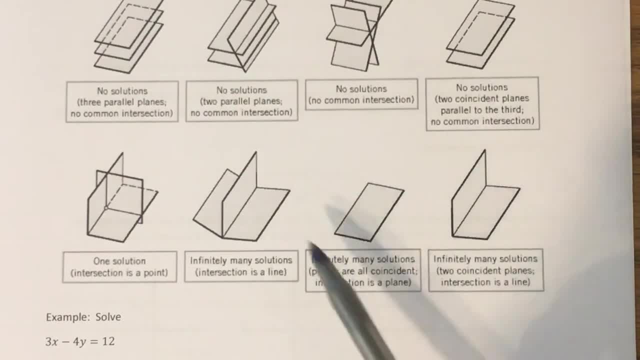 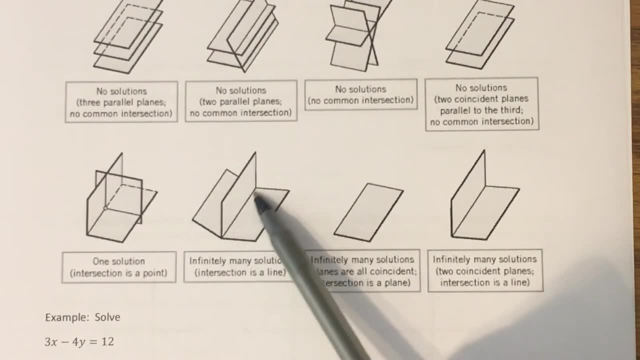 giving us exactly one solution. Okay, here's another example where we have solutions. In fact, we have infinitely many solutions. These three planes, you can see, all intersect at this line and we know that lines consist of infinitely many points. So all of the points along this line would be a. 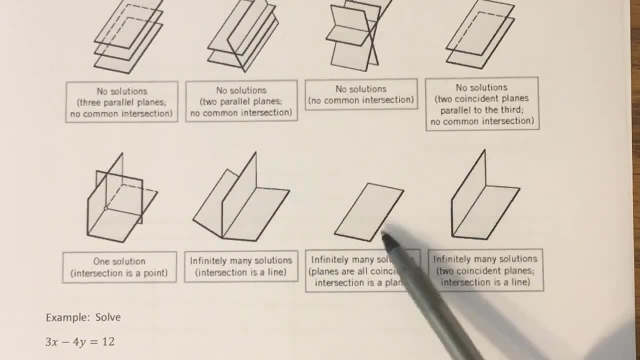 solution to the system of equations that this represents. Here's another case: All three planes coincide, which means every point on any of those planes would be a solution. And then here's a similar case. is what we have here? It's actually kind of a combination of these two cases, So 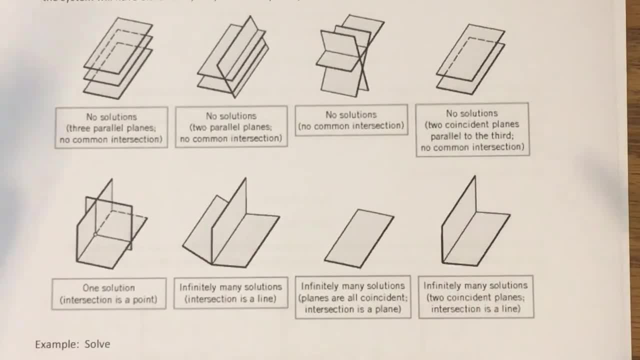 even though we can break this down into all these different configurations, we still seem to only have no solutions at all, exactly one solution, or infinitely many, And what we're going to prove later on is that this is actually going to be the case for any. 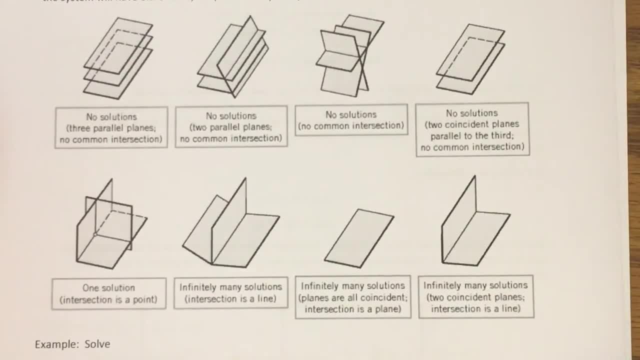 system of equations, any m by n system of equations, a system of linear equations, specifically. That's important. Whether it's a 4 by 4 system, whether it's a 10 by 20 system or whatever else you can imagine, you will only ever have no solutions at all. 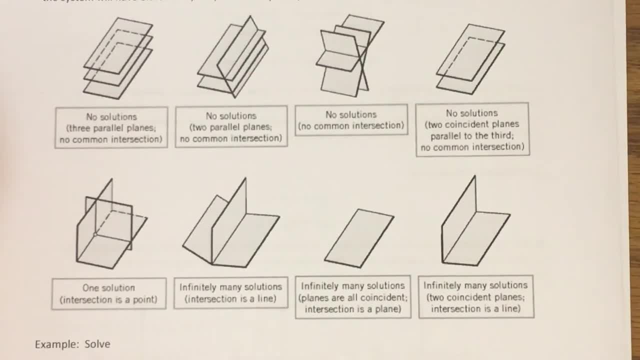 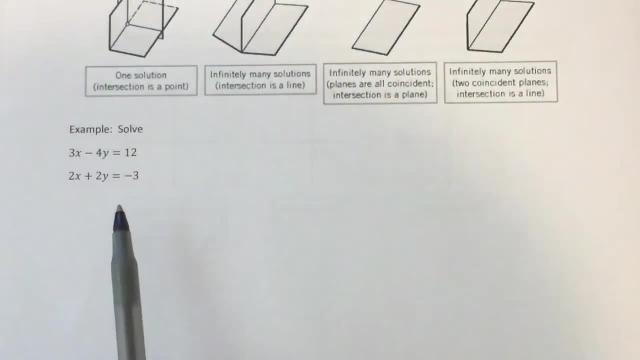 one solution, or infinitely many, Okay, so let's start looking at some examples to sort of see this happening. So, to begin with, we want to solve a simple two by two system, And this is going to be a review from algebra: how we 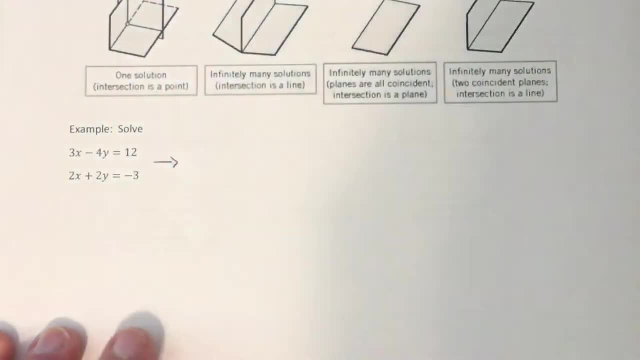 do this. So if I want to solve this system of equations, we can use an approach called elimination, where I want to eliminate one of the two variables in this system in an attempt to solve for the other variable. Notice, for example, if I were to multiply. 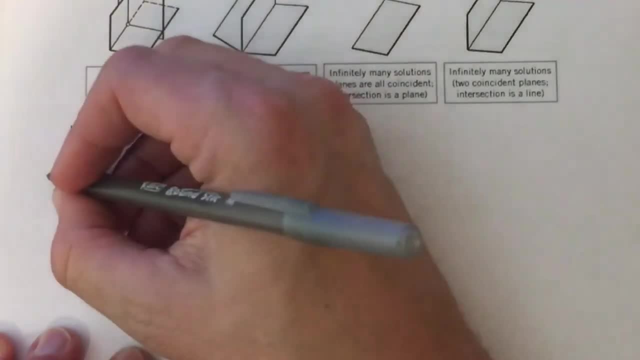 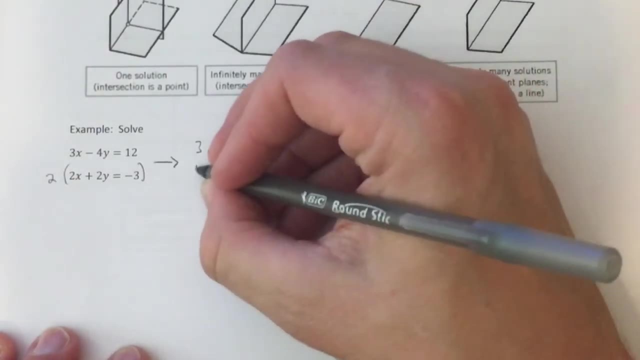 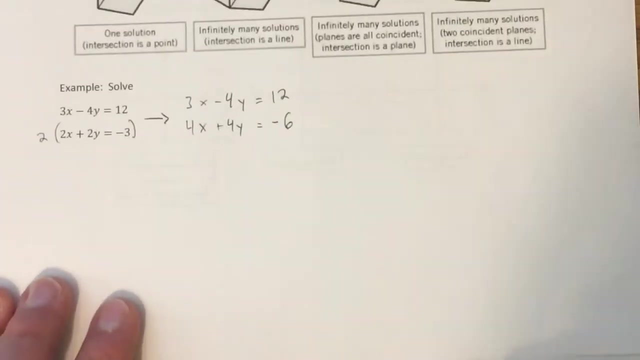 this second equation by two, then my system of equations looks like: 3x minus 4y equals 12. And down here I get: 4x plus 4y equals negative 6. If I were to then add these two equations, 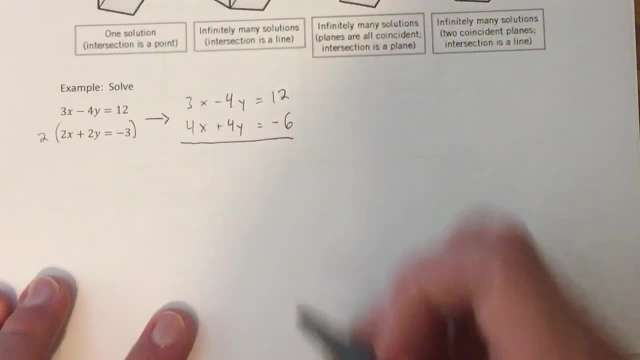 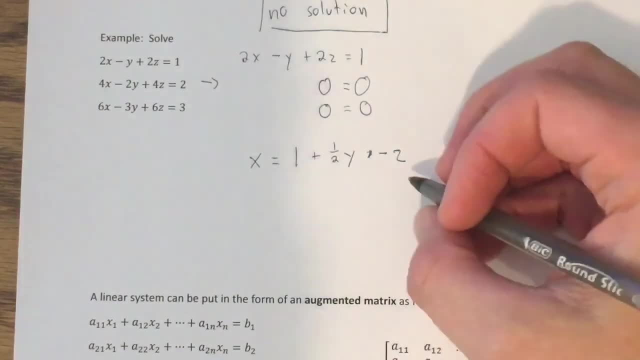 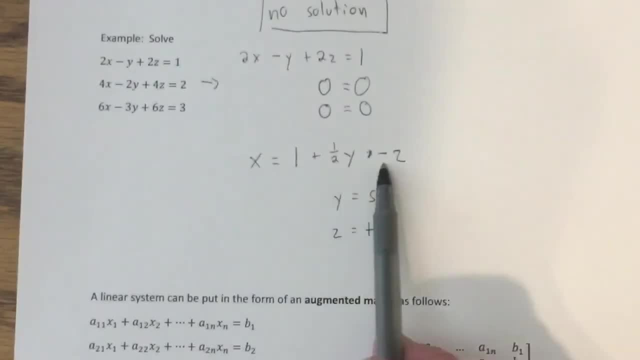 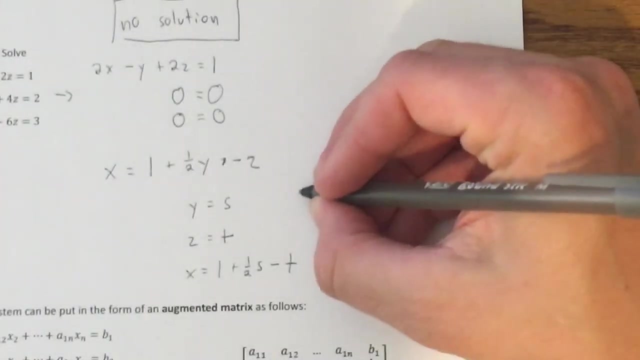 parameter t. then substituting these parameters into this equation tells me that x is equal to 1 plus 1 half s minus t. I can put all of these in the form of an ordered triple, making sure x comes first. so 1 plus 1 half s minus t, y comes. 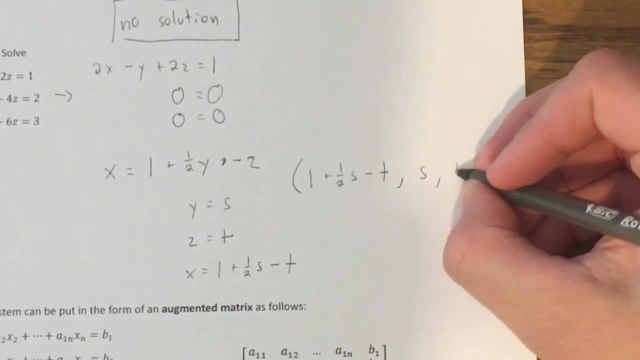 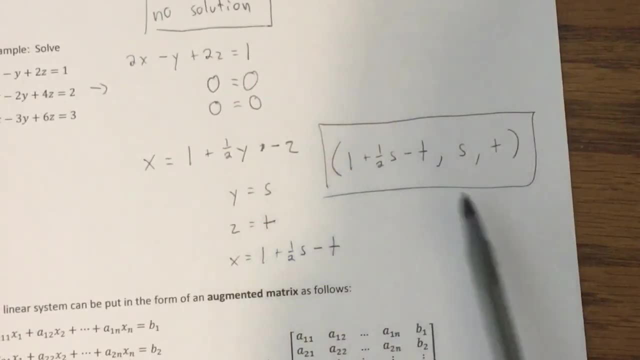 next we define that to be s and then z comes. last we define that to be t. This is called a parametrized solution set And the way we interpret this notice as an ordered triple. again, if I plug any number I want into the s's and then any, 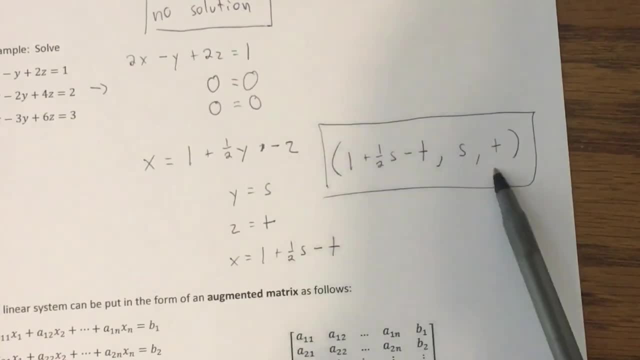 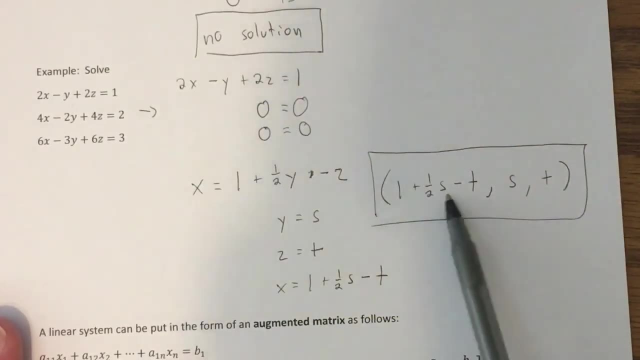 other number I want into the t's. the resulting order will be a solution to the system. I encourage you to to play with this a little bit. Pick some values and plug them in for the s's and the t's. Make sure you're plugging the same number in for both s's and then whatever number. 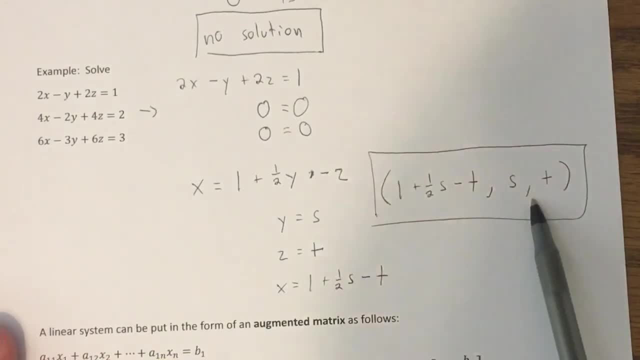 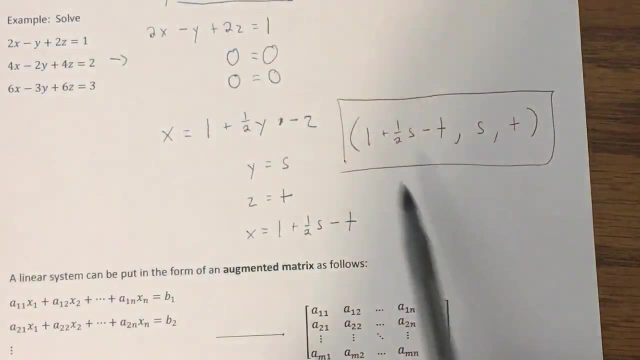 you choose for the t's, it's the same number for each one. Do that and then check and see if it actually does satisfy these equations. okay, But this is better than writing infinitely many solutions, because it's telling us what the solutions look like. This is an extremely, extremely important process.